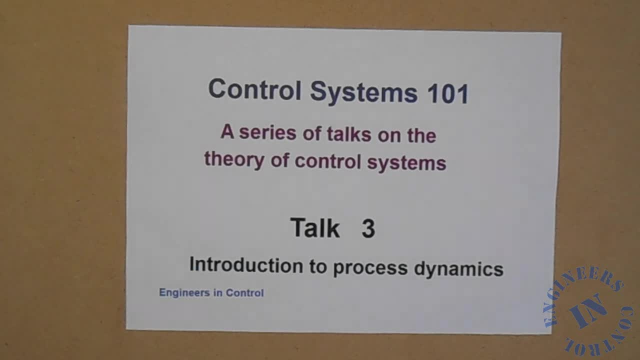 Hello, this is Paul and Dave again. This is the third talk in our series, Control Systems 101.. Talk number three is a basic introduction to the dynamics of processes, usually referred to as process dynamics. Most control processes are electrical or electronic, mechanical, fluid flow or heat control. There are 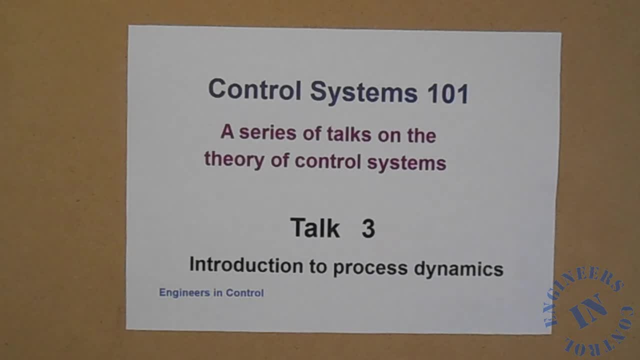 some others, such as pH control. What it is really important to understand is that all dynamic processes behave in the same way. I find it ridiculous that at university, electrical, mechanical, fluid dynamics and thermal dynamics are taught by different people in different disciplines, in different classes And 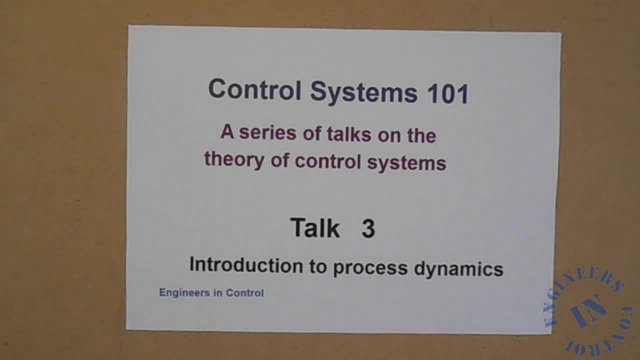 what is worse is that each of those academic disciplines use different processes, Different concepts and terminology to describe processes that behave in an identical way. Process dynamics works exactly the same for all processes, including human relationships, and, in fact, financial dynamics work the same way as well. What we are going to do in the next few talks is to treat the 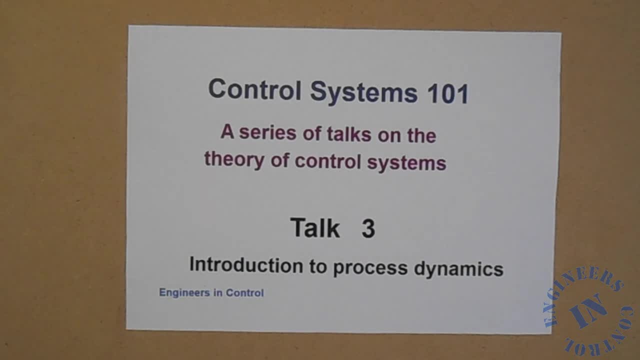 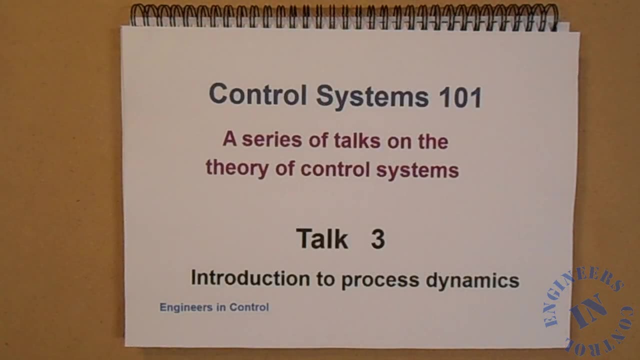 physics of each discipline, as though they are all identical. Fundamentally, there are four types of energy, which all follow the two laws of thermodynamics: 1. law of conservation of energy: Energy cannot be created or destroyed. it can only be converted from one form to another. 2. energy eventually becomes dissipated out. 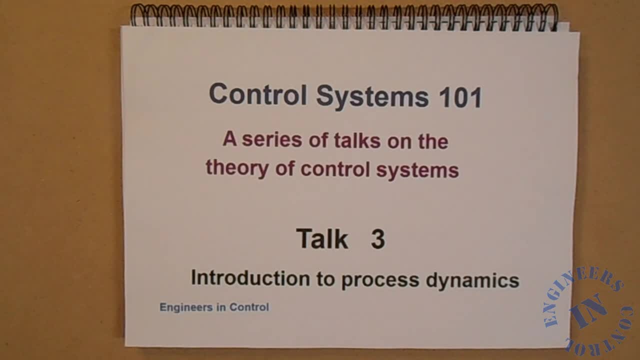 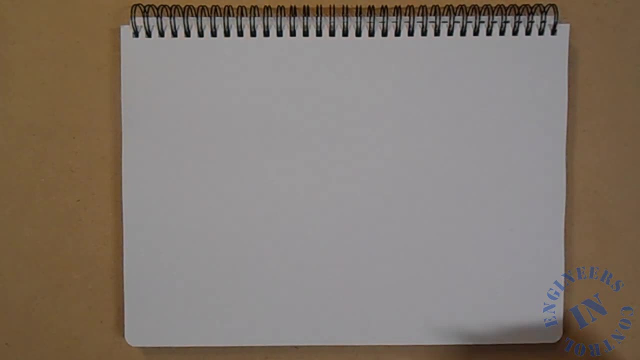 into the universe and then adds to its entropy. That is a very, very important principle, which is one of the most important things. Thank you universe. and I tend to think of these four basic types of energy in this way, so I just- I just draw this diagram. I've got four types of energy. here is a. 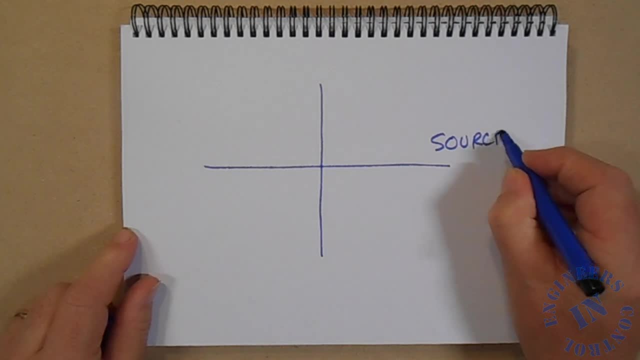 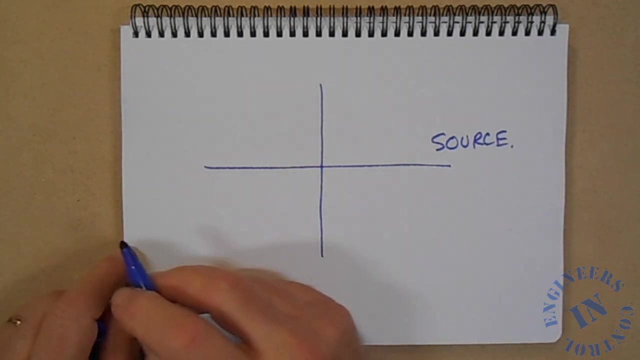 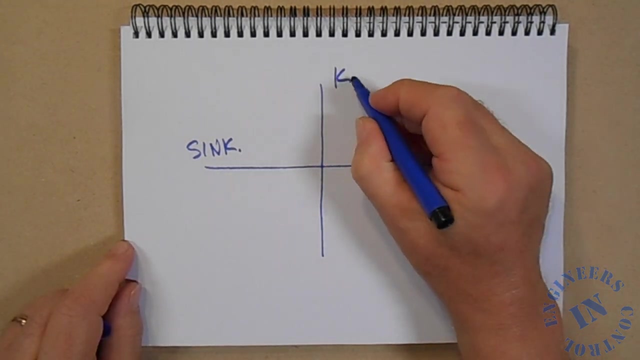 source of energy in electrical terms might be a battery, some kind of power supply, in mechanical terms, an engine and so on. and then we have a sink of energy. in electrical terms, that's a resistor. it absorbs energy. in mechanical terms, this is friction. we also have kinetic energy. 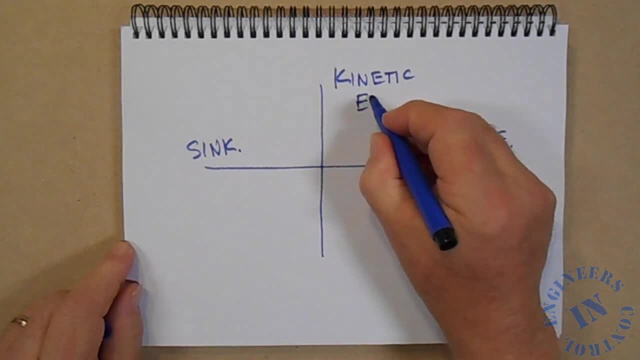 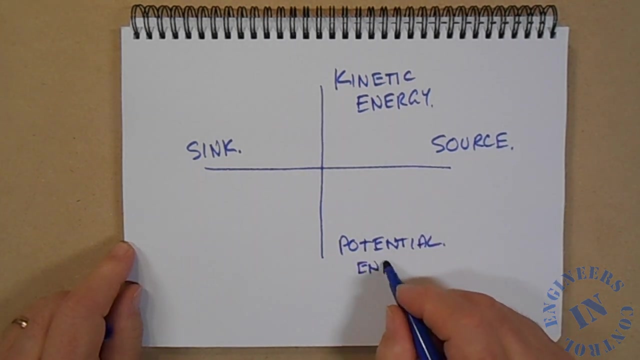 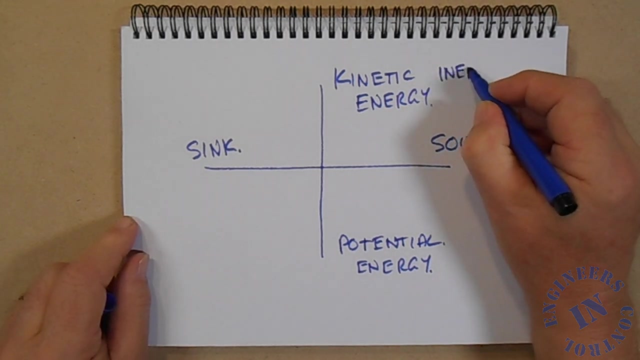 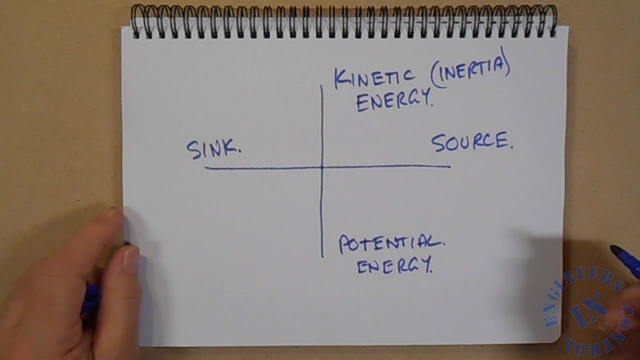 and I draw it there and we have potential energy and that's it. all types of energy in all dynamic systems. this is the sum total of how it works. kinetic energy normally would be something like inertia or inductance in electrical terms, and potential energy is some kind of storage in electrical terms. 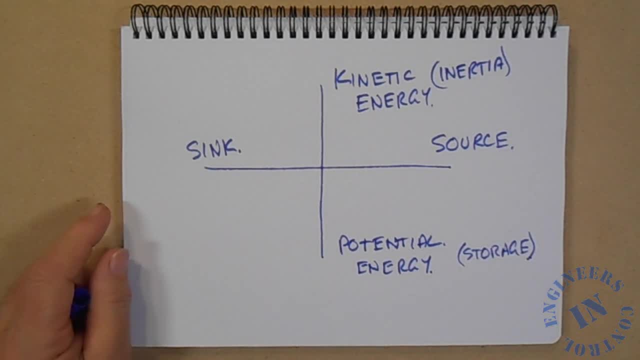 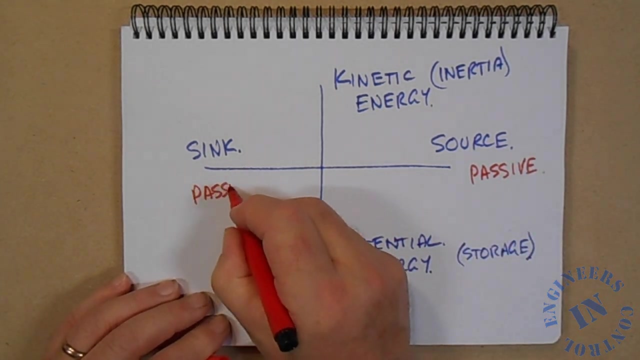 that would be a capacitor. in mechanical terms, potential energy would be contained in a spring. now it's important to recognise that the source of energy is passive and that's passive to the sink. of energy is passive A resistor. in electrical terms. we call these reactive. 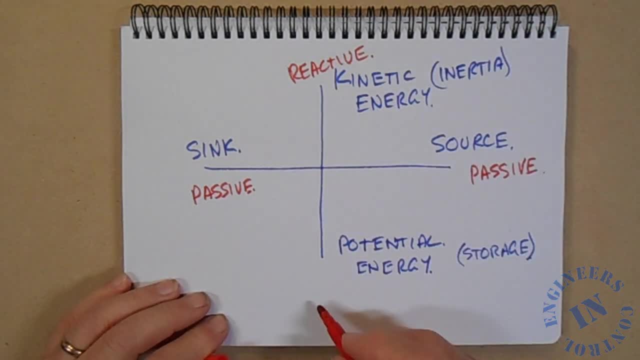 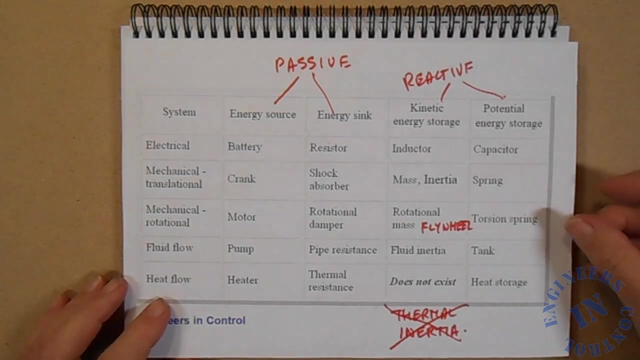 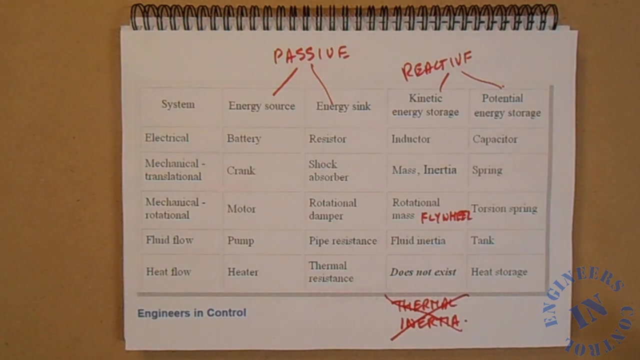 Kinetic energy will pass in this way as a vos好了. energy is reactive and potential energy is reactive. When I'm teaching system dynamics to students and people I mentor, I use this. It's a chart that I've drawn myself and I find this really convenient to explain things. 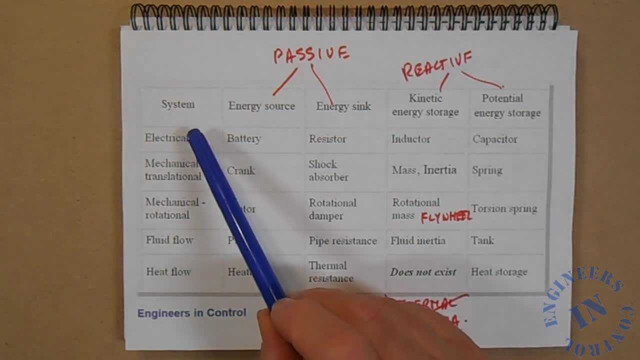 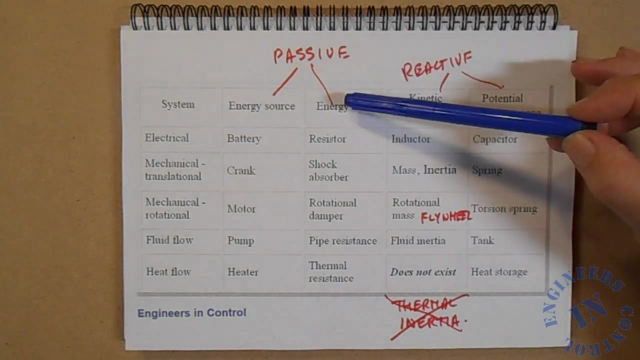 So I've got the main types of processes we find in industry: electrical, mechanical, translational, mechanical rotation, fluid flow and heat flow. And I've got my four types of energy, my source of energy, my sink of energy, my kinetic energy. 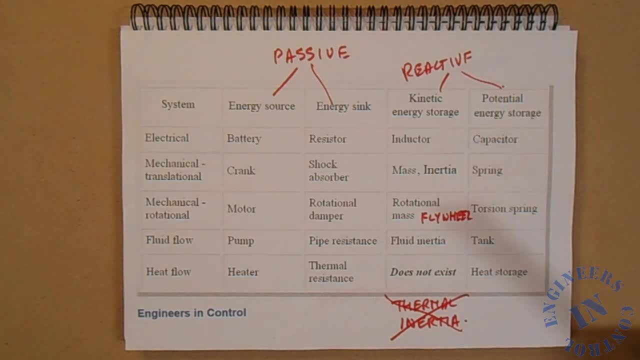 storage and my potential energy. So a source of energy, a battery, a crank, a motor, a pump for fluid flow, a heater for thermal, my sink, a resistor, a shock absorber for friction, again, friction for mechanical rotation, frictional bearings, and so forth. 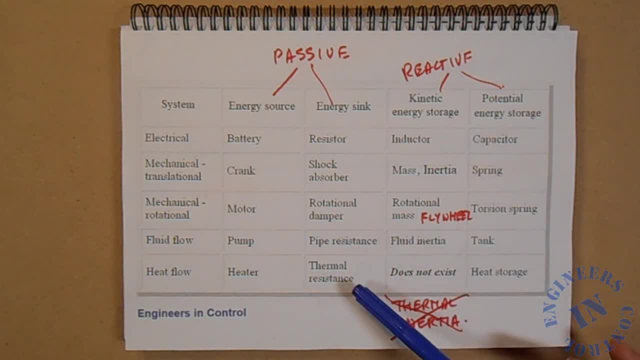 For fluid flow, the resistance in the pipe, And for heat flow we have thermal. So I've got my four types of energy Thermal resistance now, because heat is often taught by different people, They tend not to talk about resistance, They talk about conductivity. 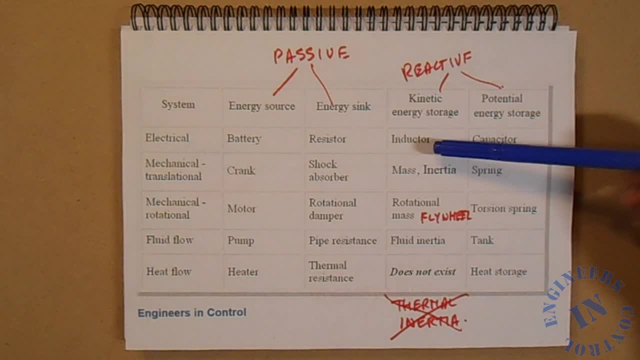 Kinetic energy storage and inductance. in electrical, the mass or the inertia. in mechanical, A flywheel has inertia. for rotational, The fluid flow. The fluids have inertia In the pipe and in heat flow. this is really important because heat does not have mass, it does not have inertia and therefore there is no kinetic energy in heat flow. so thermal inertia does not exist. you will often hear people talk about thermal inertia. it doesn't exist. what they're referring to is this one: heat storage. 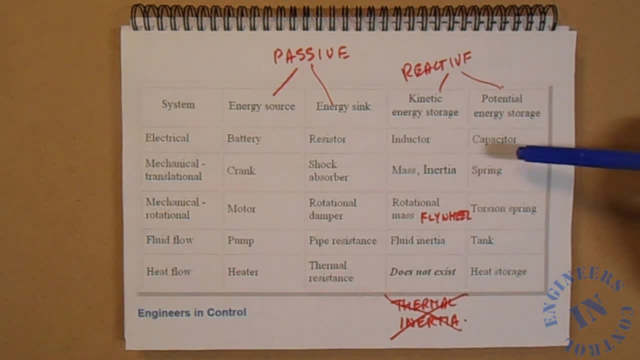 So the potential energy storage energy: In electrical it's a capacitor. in mechanical it's a spring or a torsion spring. for fluid flow it's a tank, particularly a tank up on a hill. so we have potential energy. and in heat flow the potential energy is heat storage. and once again, I repeat that when people talk about thermal inertia they're actually referring to this, because that doesn't exist.